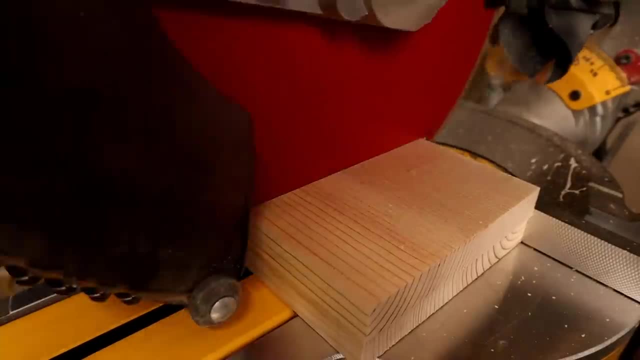 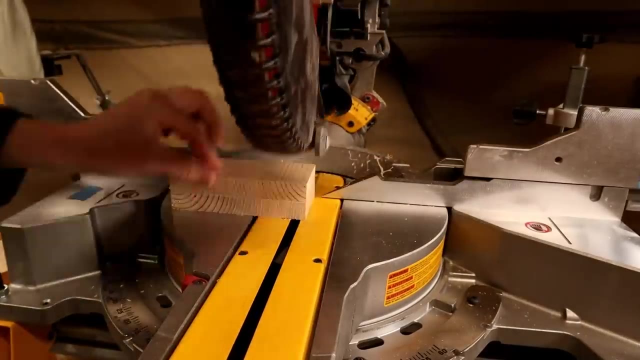 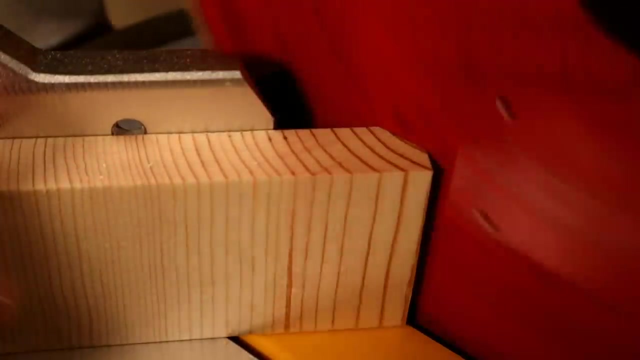 Then I measure 3 inches and make a cut. Next I shorten the pieces by about a quarter of an inch. Then, with a saw blade at 45 degrees, I clip off the corner at each end of the 2.5-inch pieces. 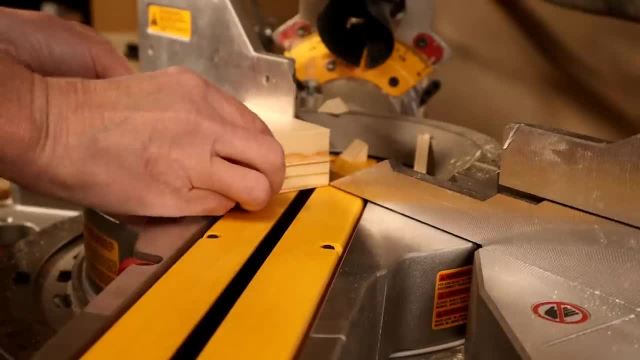 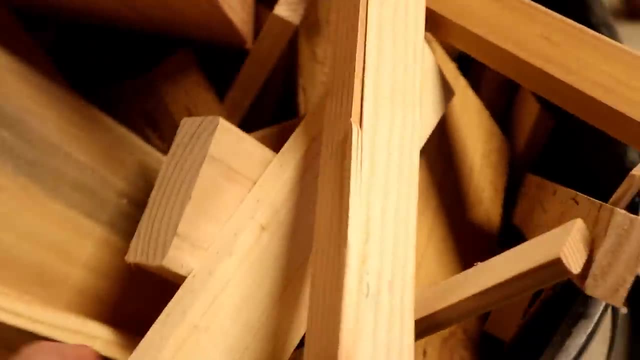 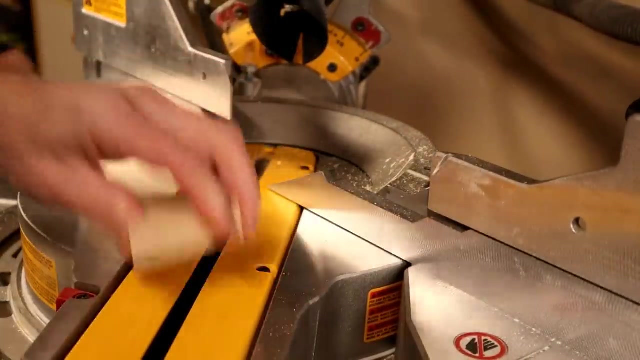 With the 3-inch pieces I cut off about 3 quarters of an inch on two opposing corners. Okay, now I grab a piece of 1x scrap wood, about 3 inches wide, cut a 45 degree from the corner and then put the saw blade back to 0 and cut that piece. There will be four of these pieces like that. 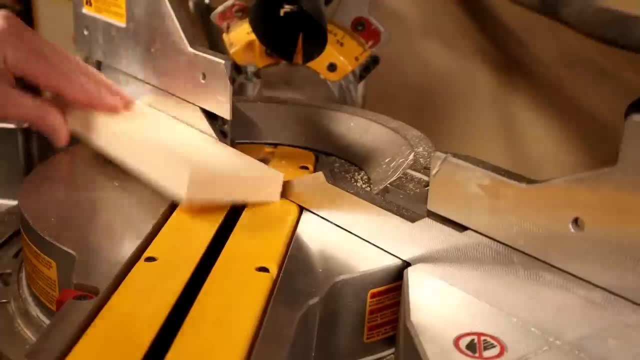 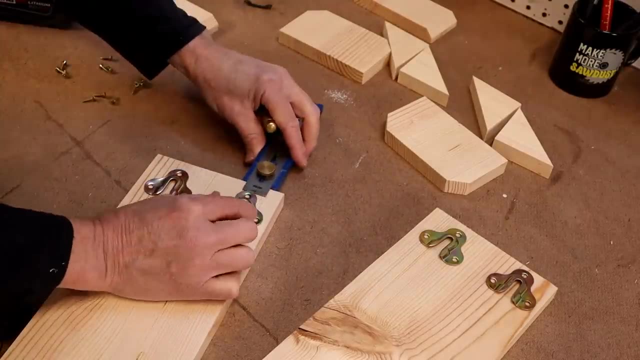 Before I proceed further, I go ahead and attach the keyhole plates. It's easier to do this now, before the other pieces are attached. Before I proceed further, I go ahead and attach the keyhole plates. It's easier to do this now, before the other pieces are attached. 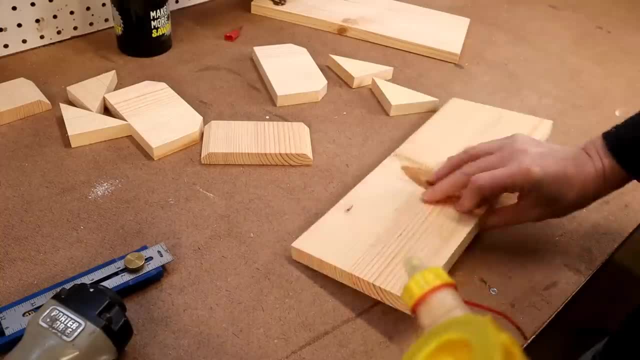 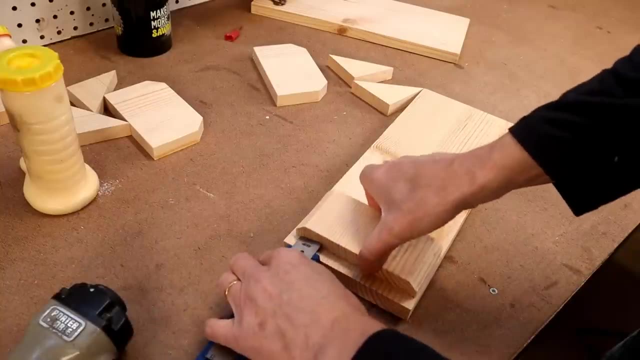 Before I proceed further, I go ahead and attach the keyhole plates. It's easier to do this now, before the other pieces are attached. Next, I glue the 2.5-inch wide piece- about 5-8ths of an inch- down and centered on one end, then put some 1-1⁄4-inch nails in. 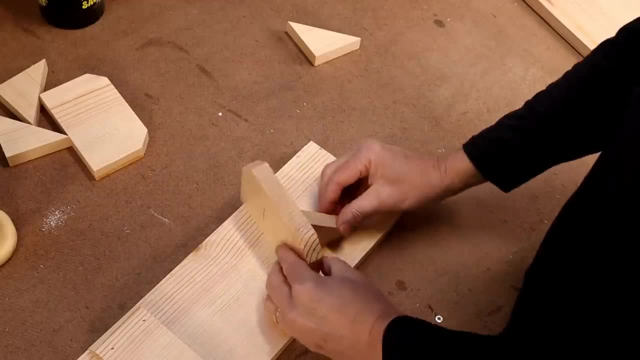 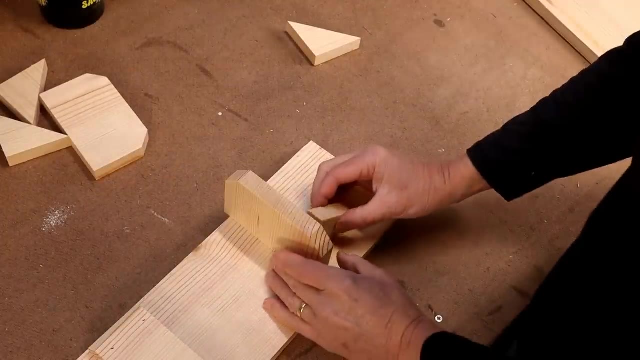 Before I proceed further, I go ahead and attach the keyhole plates. It's easier to do this now before the other pieces are attached. Now I'm attaching the 45-degree angled braces to the bottom of the 3-inch wide piece. Notice the notched corners are facing forward. 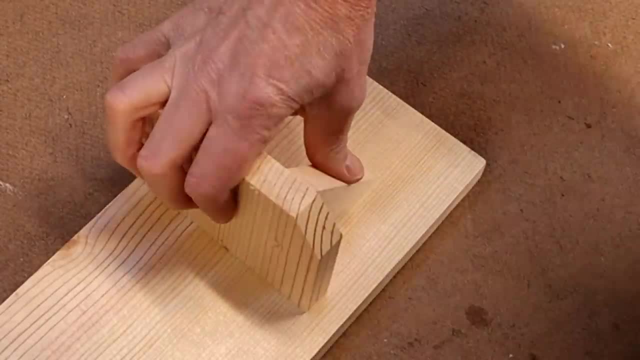 Before I proceed further, I go ahead and attach the 2.5-inch wide piece, about 5-8ths of an inch down and centered on one end, then put some 1-1⁄4-inch nails in. Notice the notched corners are facing forward. I then shoot a nail in to keep it in place. 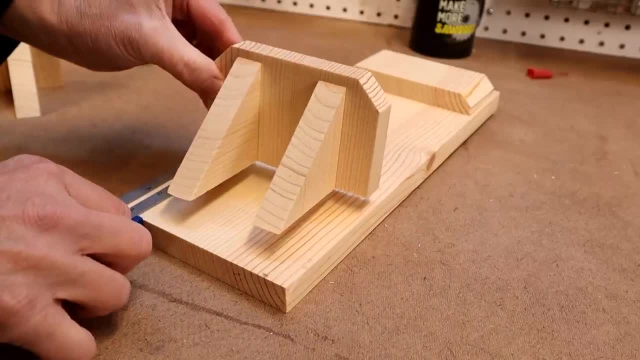 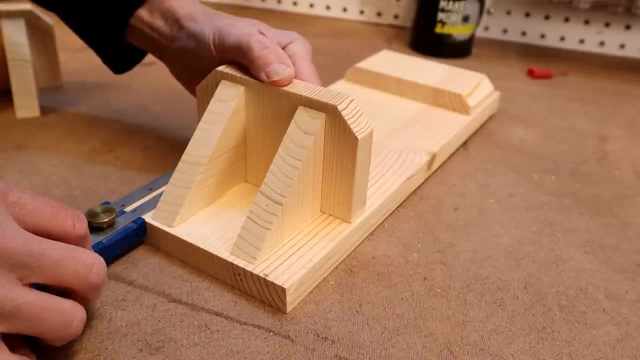 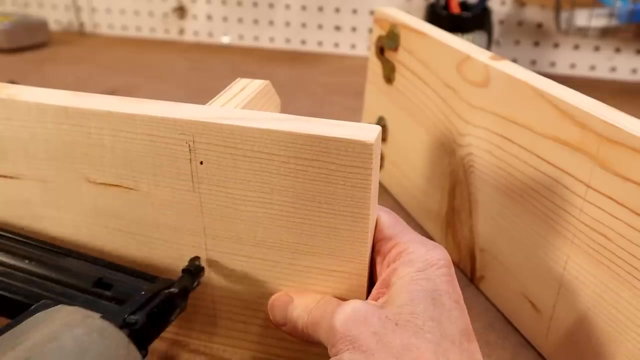 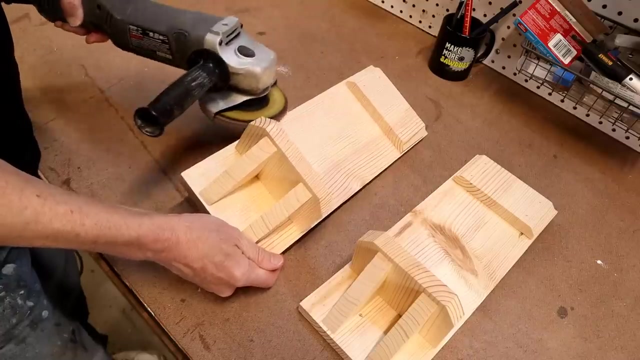 Then I glue the back edges of the braces and bottom shelf and place in position as shown. I go ahead and let the glue dry and then mark a reference line so I can shoot some nails in for extra support. Next I do some rusticating with my angle grinder and 60 grit pad. 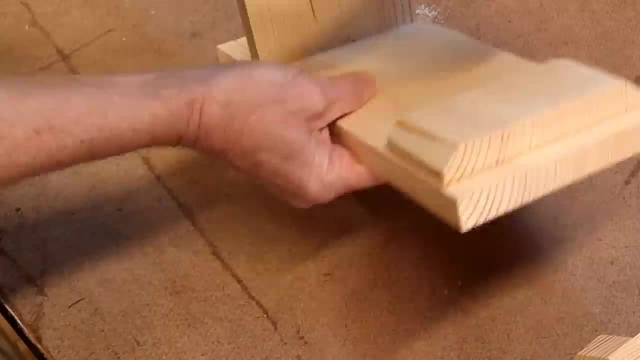 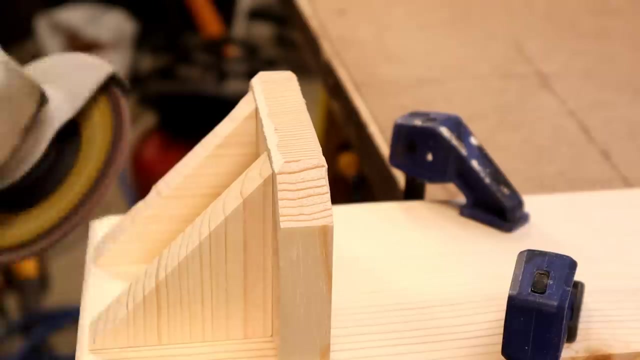 Now, these are going to be rustic pieces, so there's really no right or wrong way to bevel the edges. The important thing, though, is, if you're going to do it this way, apply very light pressure when you make contact, because the wood will grind away in a hurry if you're not careful.